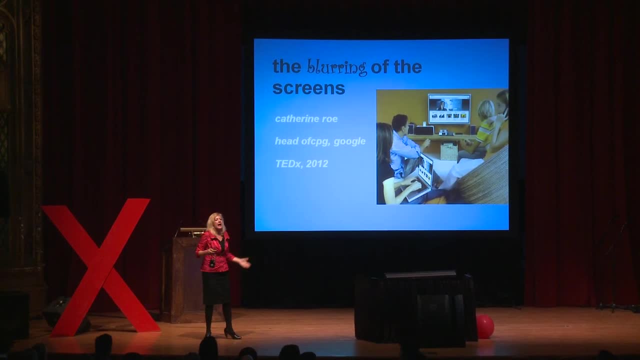 than one device. This is phenomenally different than what it was three years ago. This dramatic shift in the devices that we have available for us is: we haven't seen this type of shift in the consumption of media behavior since the 1950s. quite honestly, when the TV first turned on. 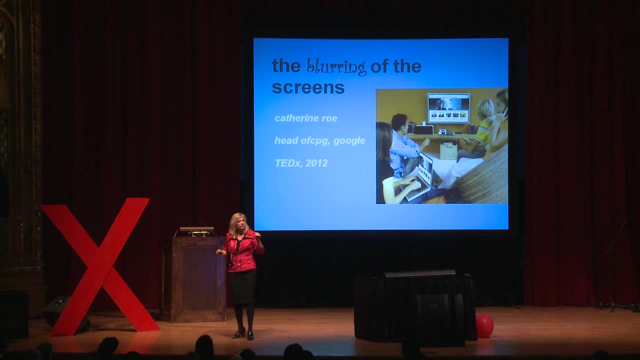 Most of you in this room have always had the TV. In fact, you don't have the luxury of the time where you actually had to get off the couch to go change the channel. Because of this dramatic shift, we're consuming media so much differently than we have in the past. 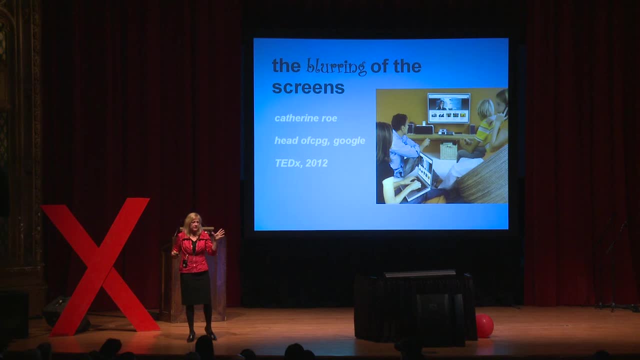 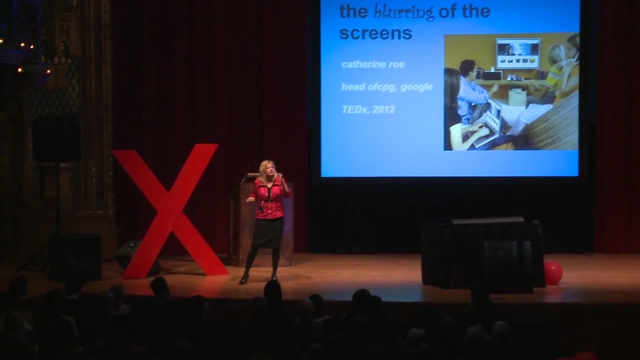 This is really important to marketers. I work with a lot of CPG companies, consumer packaged goods companies, so the Procter & Gamble's, the General Mills' of the world, and they have a lot of different types of products. I always like to tell them: your consumer. 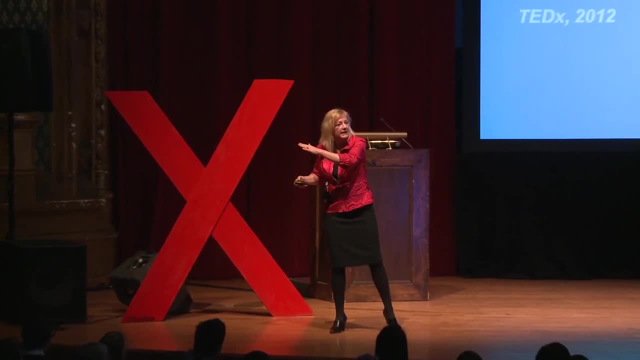 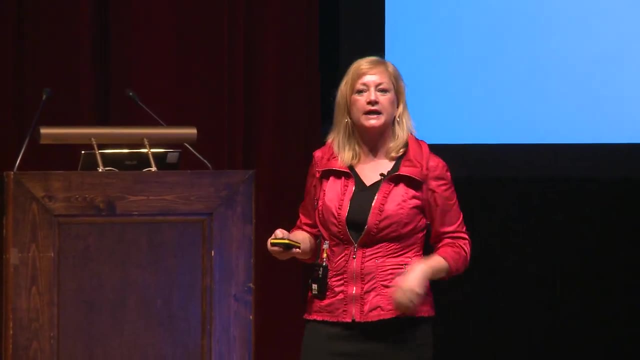 has already left the building as far as where they're getting their media and they don't really care if you follow them or not. Our advertisers need to think differently about how they market to today's consumer, when we're getting our media across a bunch of different. 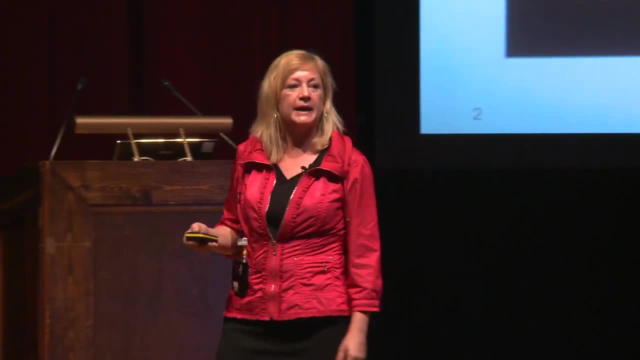 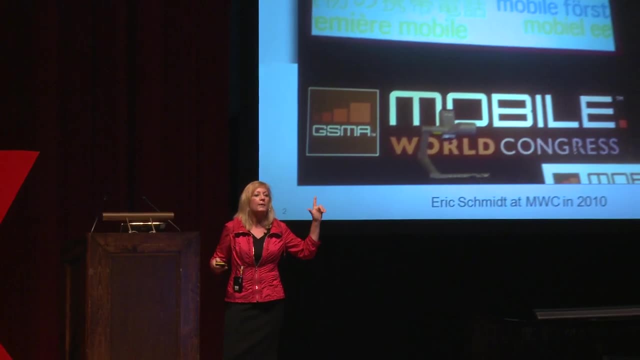 devices. This is Eric Schmidt, who is our Google chairman. This is a conference that he spoke in back in 2010.. He put up this slide called Mobile First. Why Mobile First? Google makes more than 90% of our revenue on those little text ads on Googlecom that. 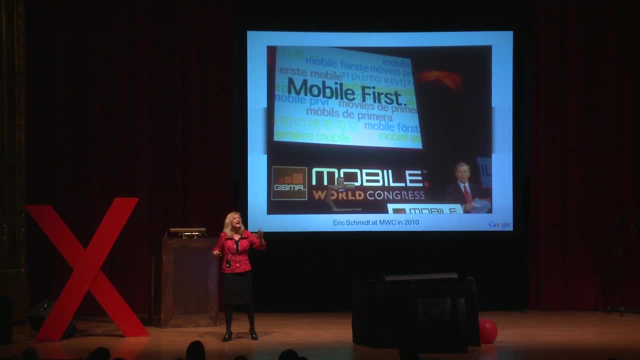 people say they never click on, but somebody is clicking on them. Anyway, if we don't have the vision to look ahead, to know that our consumer's habits are changing onto mobile, then that's going to hold us back from continuing our progress as a company. 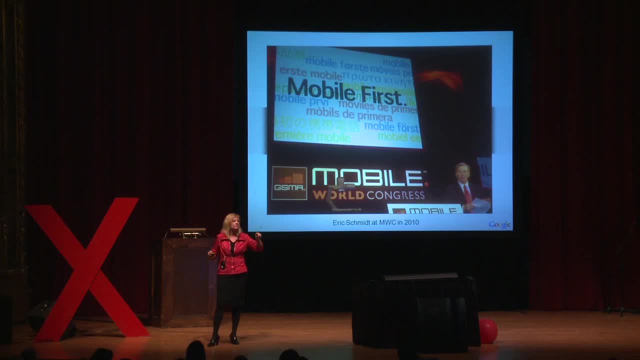 When he says Mobile First, that means that every product that comes out of Mountain View or Google, whether it's an enhancement of Google Maps or the new Google Drive, the first thing they ask is: what is the mobile application? Because we can't continue just. 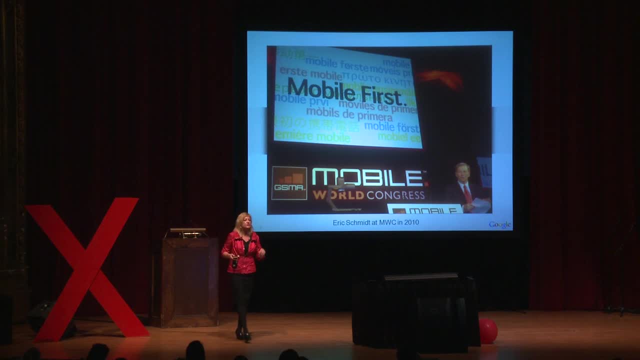 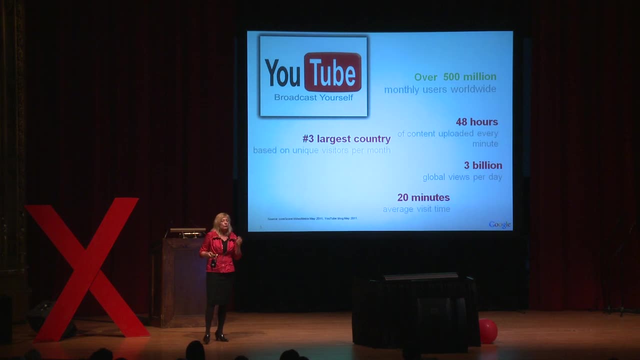 to create things for the desktop when the consumer has so many other devices at their disposal. Google also owns YouTube, which is the largest video platform, and why this is so important- especially when we put on the lens of a marketer- is that in 2015,, more than 80% of the time spent on the Internetwas. 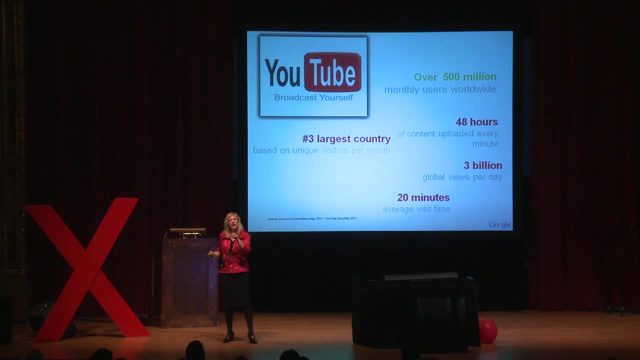 Google that more than 80% of the time spent on the Internet was to be installed into Facebook will be watching video. YouTube alone commands more than 10% of all the broadband. because of so much video watching- And this is important, because your habits have changed- Video is on. 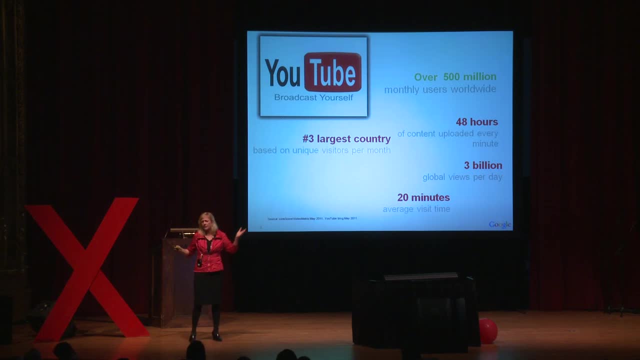 demand. It's no longer I have to be home at 7 o'clock to watch the Big Brother episode, right? You watch it whenever you want, on whatever device you want. In fact, most of you in this room will never own a Comcast cable or an ATT cable subscription. Why You've got Netflix. you've 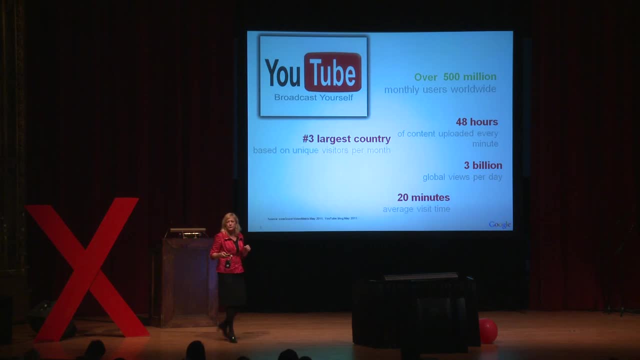 got YouTube, you've got Hulu. Who needs to have a cable subscription? You'll never have that intimate relationship that I have with my Comcast provider, where I unplug the box, plug it back in, sit there for 45 seconds of awkward silence and then they finally dispatch a Comcast guy to my 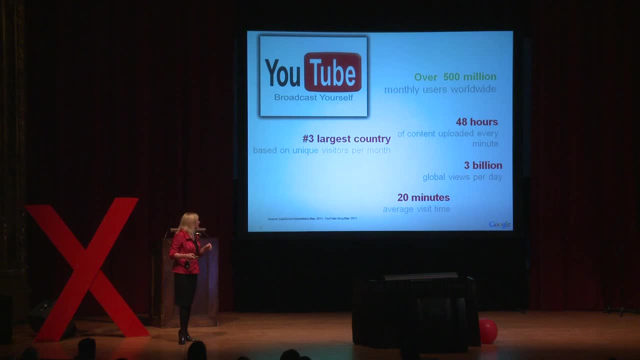 house, But it's good You'll miss it. YouTube: Over 500 million monthly users. If YouTube was a country, it'd be the third largest country. 48 hours of content uploaded every minute, 3 billion global views per day and 20 minutes on. 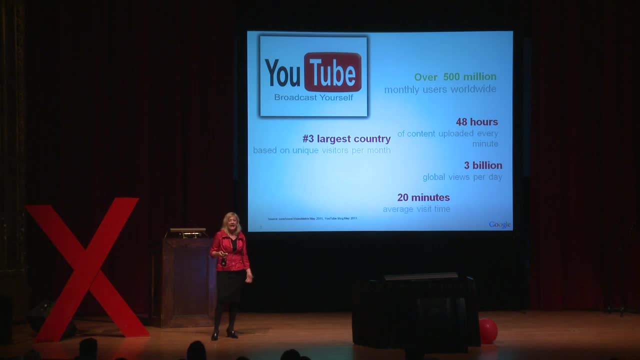 average spent there. People get to YouTube and they're having a good time right, And it's not just cats on skateboards anymore. There's a lot of good quality talent out there, And so one of the things that we at Google work to do- and I have some colleagues in the audience here- we educate. 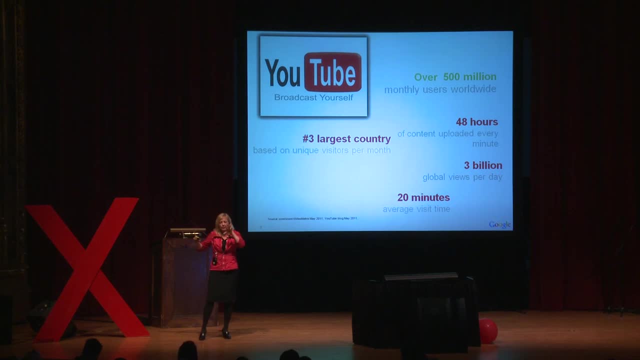 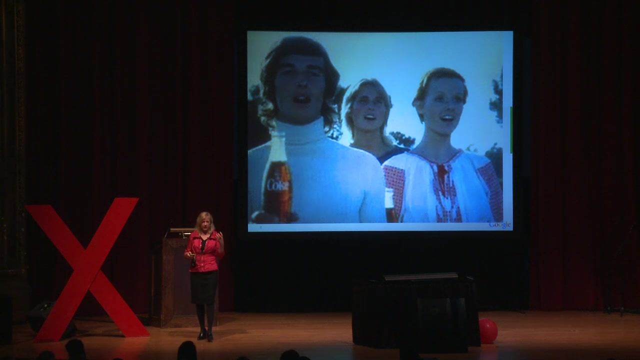 our marketers. How do you adapt your programming when you're so used to TV, for the most part as a means to get to your consumer? How do you adapt in this world? And so what we did was a project called Rebrief. Here we go, And this was a project to help our marketers start to think differently about if 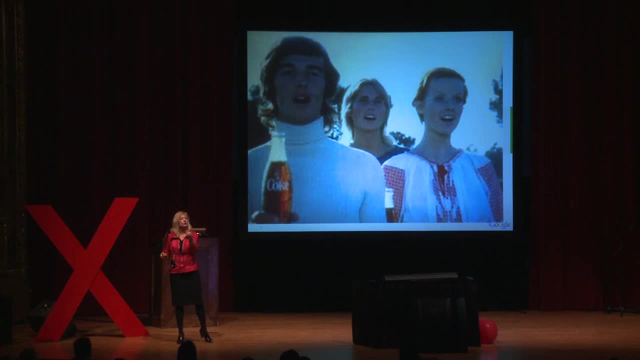 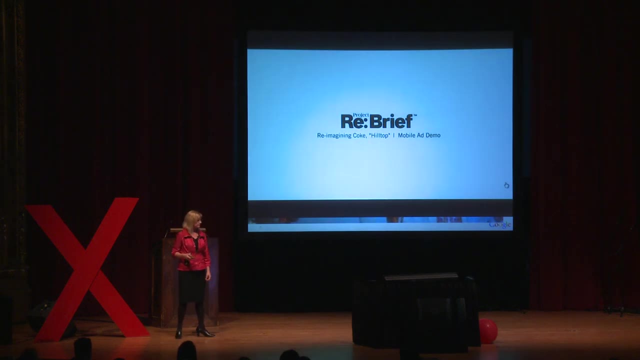 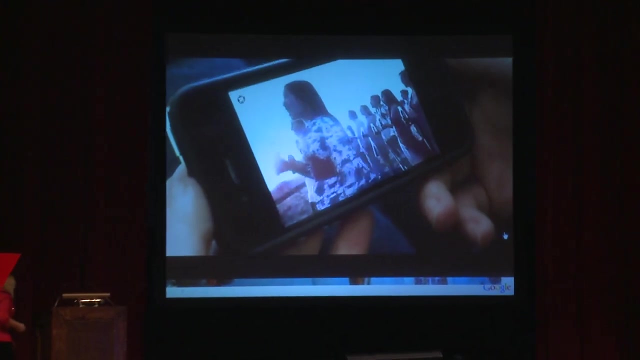 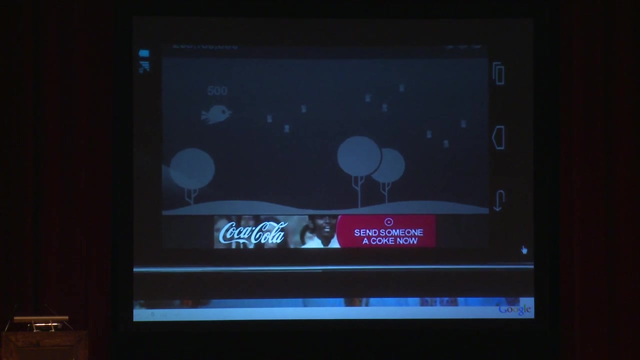 you looked at iconic campaigns from the past. what would those look like in today's world where you have this technology at your disposal? In Project Rebrief, we've reimagined Coca-Cola's classic hilltop commercial for a modern audience in the digital age. In the spirit of the original ad, it allows users to connect with strangers by 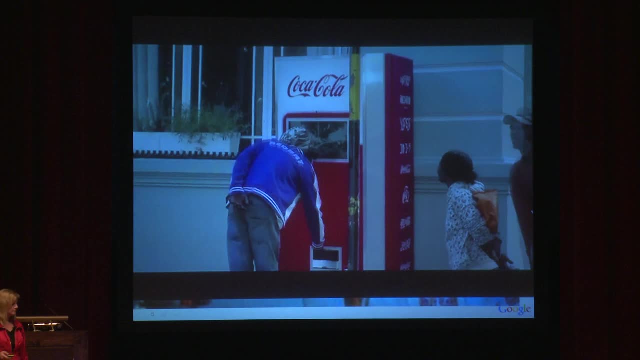 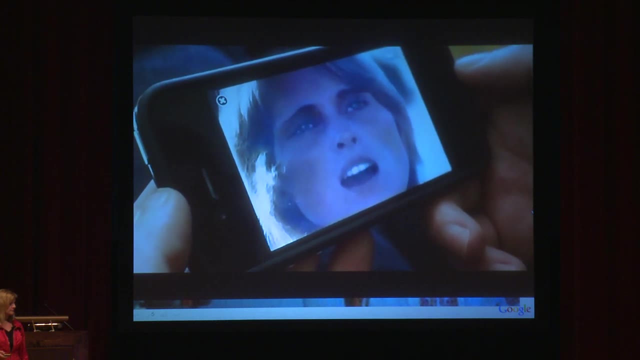 sending a Coke around the globe to an unsuspecting recipient, making the world feel just a little bit smaller. The ad can be experienced on mobile phone apps in Google's AdMob network across iOS and Android devices, Made possible through AdMob-rich media ads coupled with custom-designed vending. 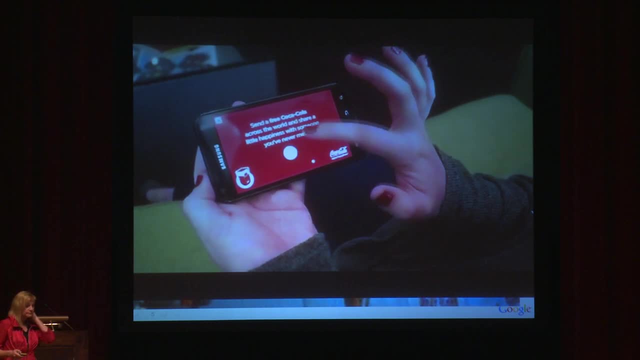 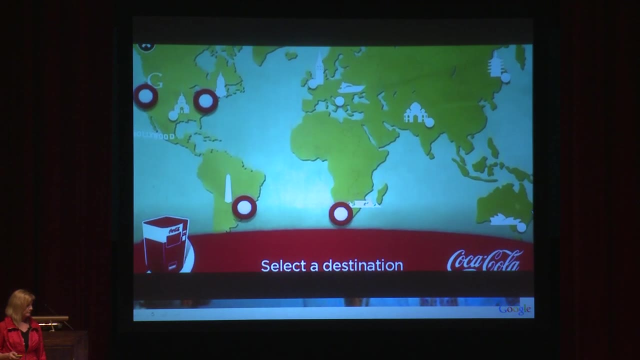 machines. viewers can truly buy the world a Coke with a few taps on their mobile phones. A viewer can decide where to send a Coke by selecting one of many machines located around the world, from New York City to Cape Town to Buenos Aires. They can then add a custom. 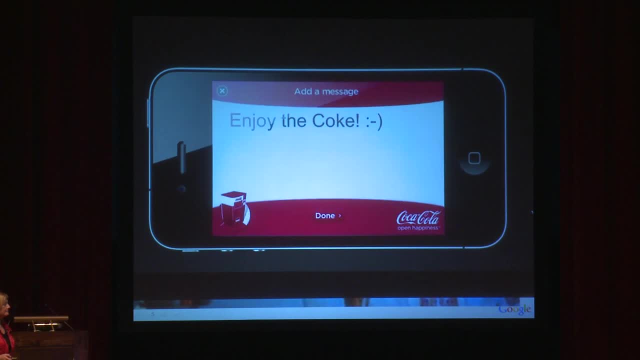 text message to personalize their Coke delivery. Google Translate converts these messages on the fly, breaking down the language barrier across countries. A dynamic video with Google Maps, Street View and composite motion graphics shows the Coke's journey from the viewer's current location to the vending machine across the globe. 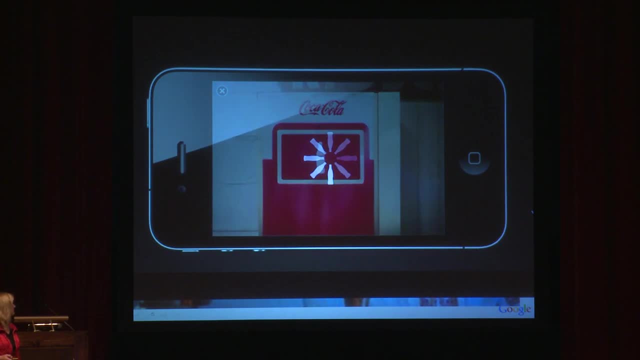 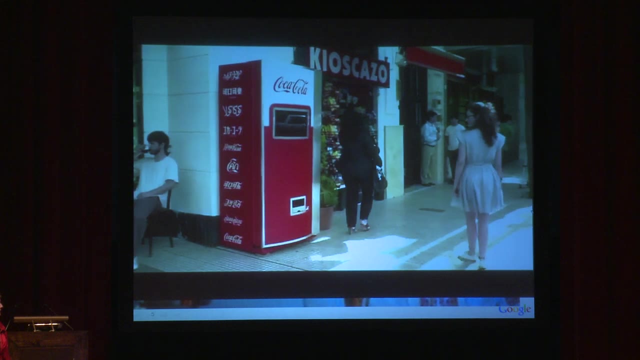 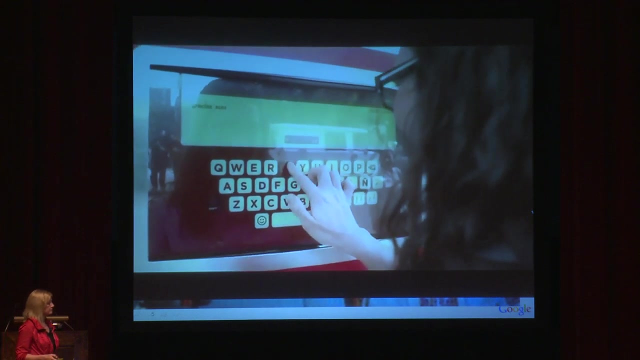 Users can then wait for confirmation of their Coke's delivery or enter an email address to be notified later. Once the Coke is delivered, recipients are not only treated to the generosity of a stranger thousands of miles away, but they can also say thanks by sending a message of their 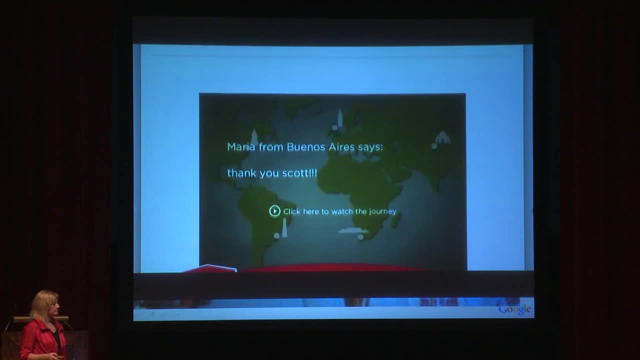 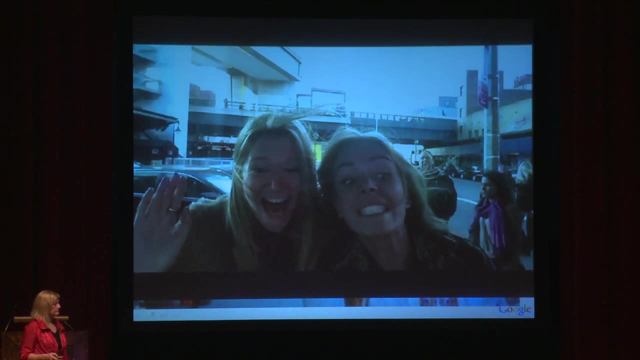 own back home. This way, they can send a message back to the user. That message is then delivered to the user's inbox, where they can read the note and view a video clip of the recipient's surprised reaction upon getting a free Coke. 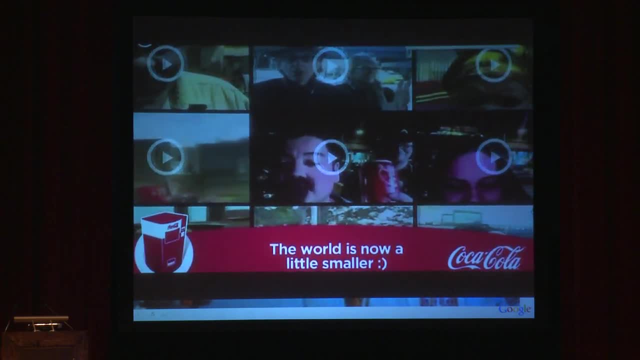 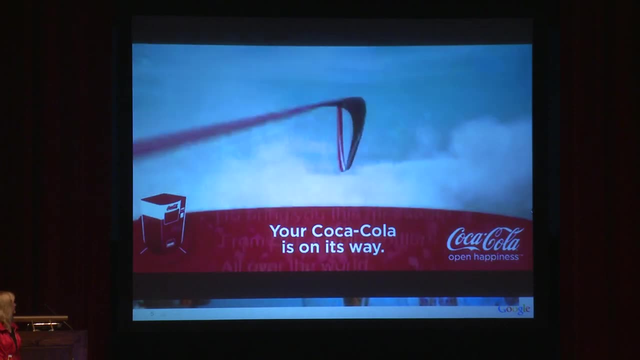 A gallery showcases some of our favorite shareable exchanges between people around the world connecting over a can of Coke. Today's technology allows us to make good on a promise Coca-Cola made over 40 years ago and lets users buy the world Coca-Cola- the best Coke I've ever had. 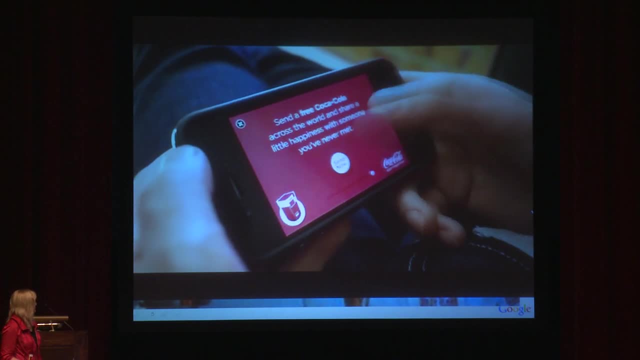 Today's technology allows us to make good on a promise Coca-Cola made over 40 years ago and lets users buy the world Coca-Cola- the best Coke I've ever had. Coca-Cola- the best Coke I've ever had. roll the coke from the palm of their hand. 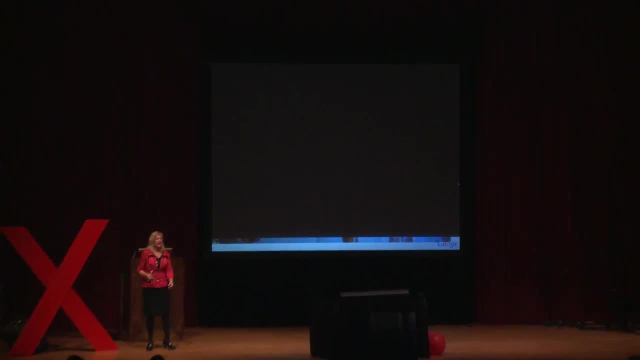 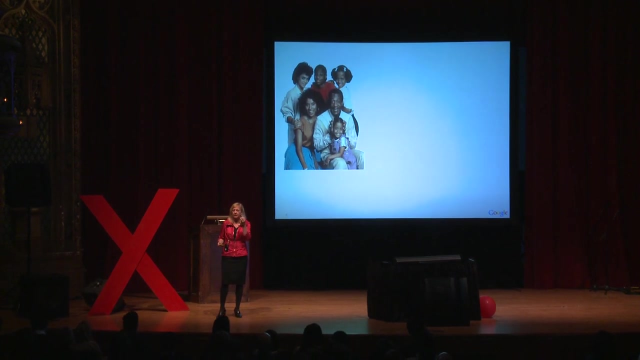 Isn't that cool. So it's really thinking differently about how to use technology, And so a lot of advertisers right now are thinking, well, oh my God, I don't know how to make that shift, But the progressive ones are having a really good time at it. 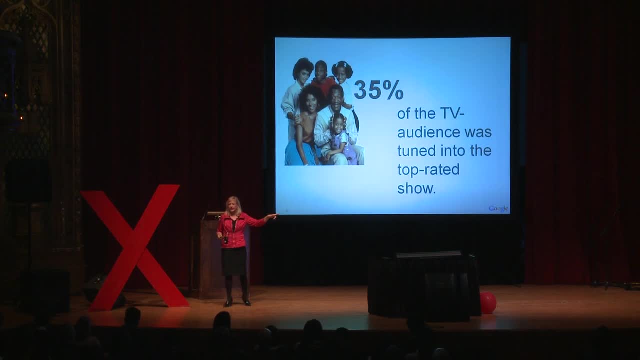 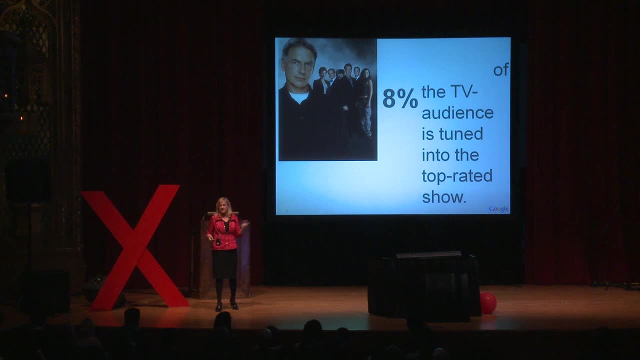 So let's take a look back: 35% of the household back in the 80s. if you were a marketer, you knew you could catch 35% of those people if you advertised on The Cosby Show. Today's top ad, or NCIS, only gets 8%. 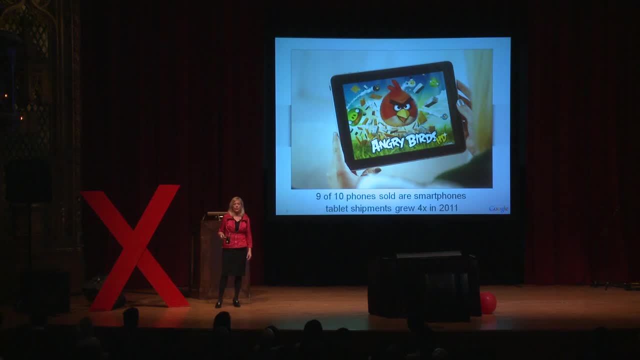 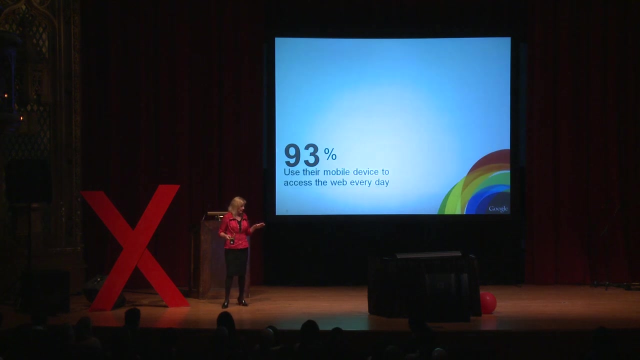 The market is so fragmented. How do you reach those folks? today, Angry Birds, 9 out of 10 phones are sold, with smartphones and tablets are up four times 125 years of Angry Birds played every single day. That is a lot of angry people. 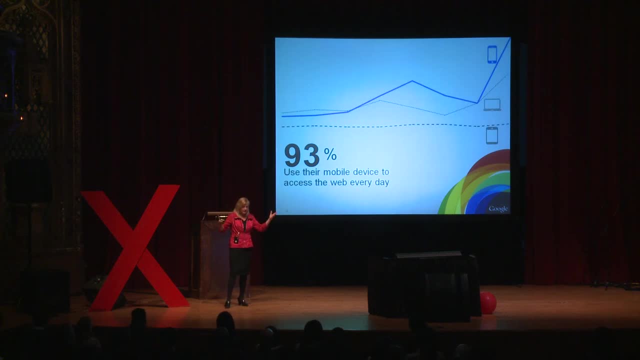 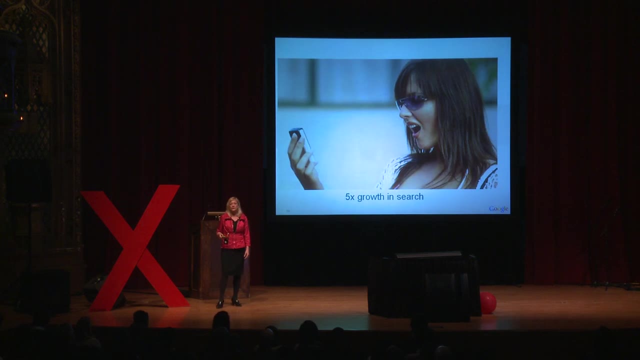 So 93% of us with our smartphones. we use our smartphones to get on the internet every single day. Five times growth in search. So again, mobile search is growing dramatically And in fact, what we're finding now is 20% of searches are now done on a mobile phone. 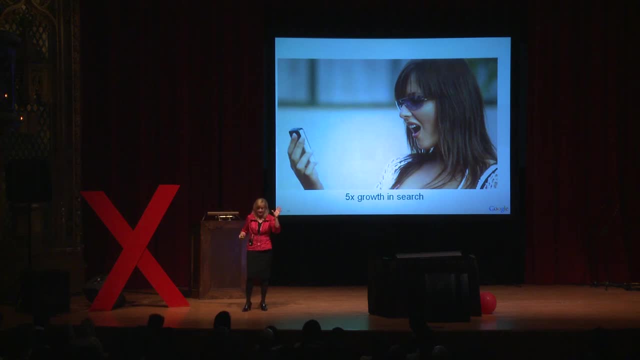 And yet we work with advertisers. I'm not making this up. We work with advertisers who say: well, you know what? Mobile is part of my 2014 plan, And I'm like you're kidding me. So 20% of the searches are coming from a mobile phone, yet you have an 800 number. 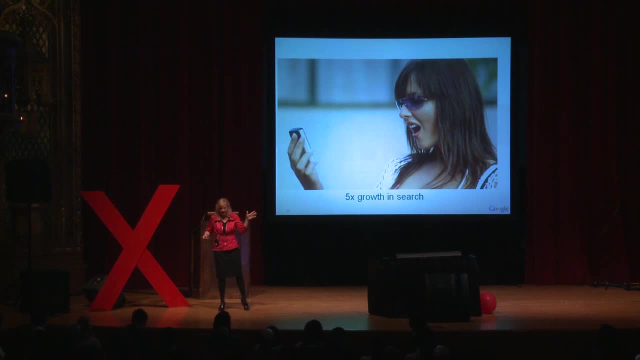 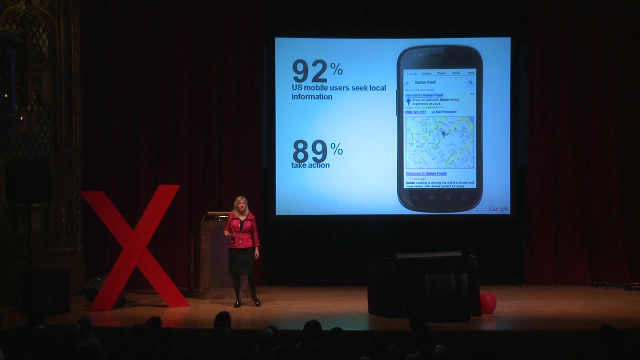 That's like saying every fifth call don't answer on an 800 number, right? So it's amazing the growth of it. today, 92% of users seek local information, So one in five searches on desktop Googlecom. it has a local intent. 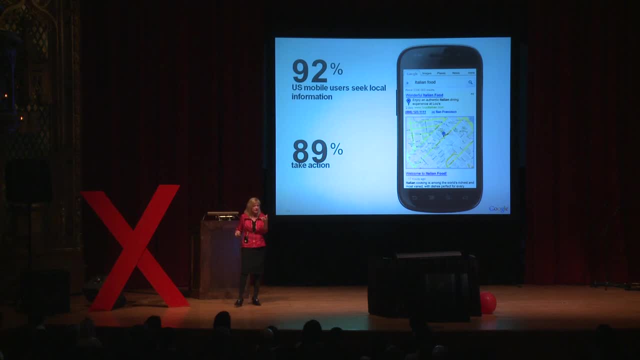 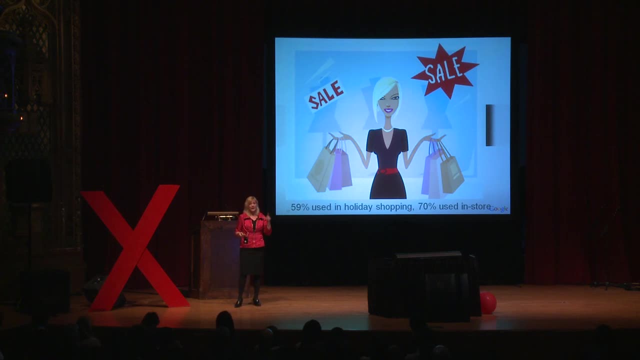 One in three on a mobile phone. Because you've got your phone, you want to know right away, And 89% of those folks take action. 59% use it in holiday shopping And more than 30% of searches on Googlecom on Black Friday came from a mobile phone. 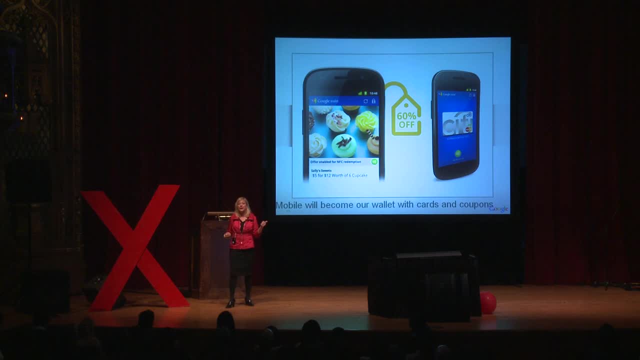 So, as a marketer, yeah, I need to be there. Mobile will become our wallet. And why is that? Our studies have shown that you will figure out that your mobile phone is missing before you figure out your wallet or your child is missing. 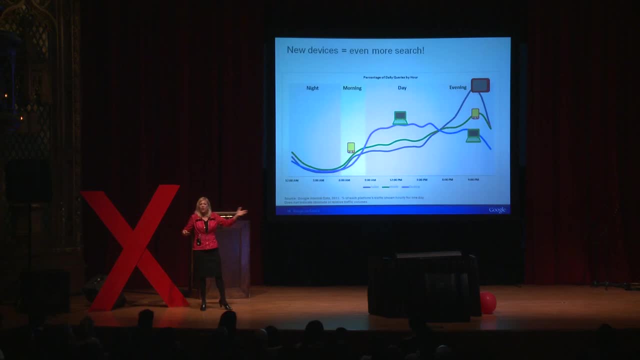 And with these new devices it actually increases because we're always connected right. So what's really interesting is this. What's interesting is the growth of tablet, especially in the evening. So again, for marketers, this means I have to figure out what my consumer is doing and make sure that I'm there to communicate with them. 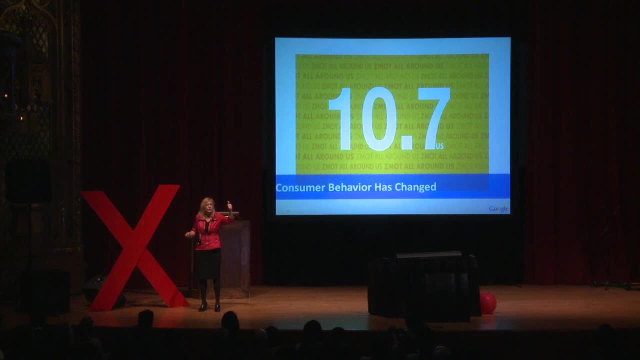 10.7,. this number is the number of references people use on average to make a purchase decision. And this isn't just what restaurant I'm going to go to tonight or what vacuum I want to buy. This is what hair shampoo will not make my hair frizzy. 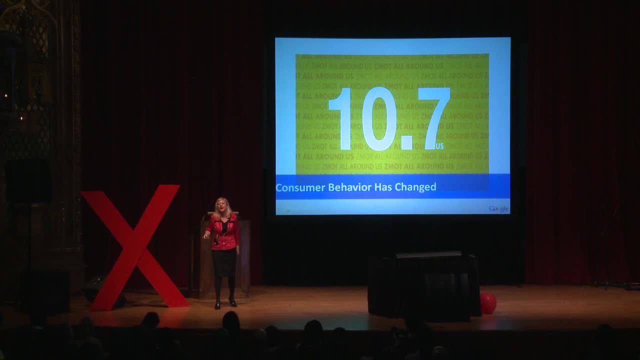 10.7 sources before they make an everyday purchase, And that's up from 5.3 a year ago. Why? Because I have it there. I want to get the best deal. I know how to do it. I have technology. 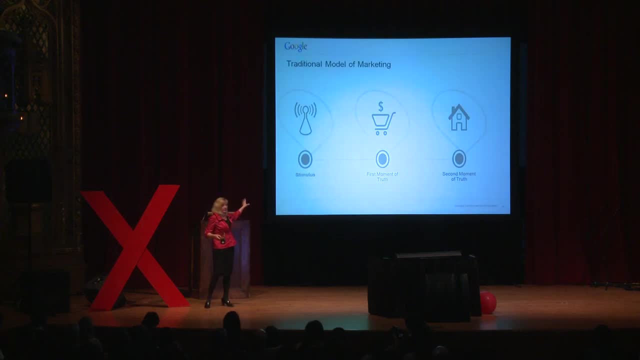 So the traditional mode of marketing was the stimulus, the TV commercial or the billboard. The first moment of truth: I got to the shelf, I found what I wanted. And then, the second moment of truth, I got the shampoo home. it made my hair frizzy or it didn't. 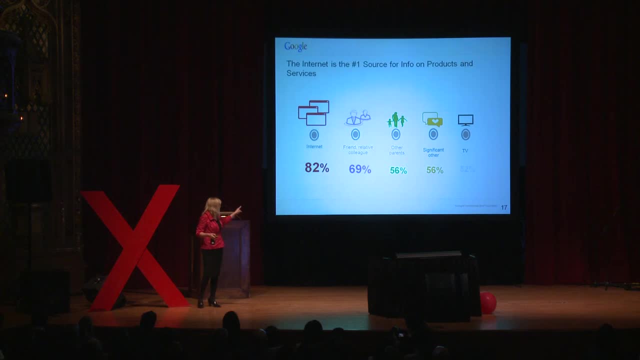 What's changed is consumer habits. Now, if you look at this, 82% use the Internet to find information right, And so what that's created is what we call this new zero moment of truth is this moment we're looking at the computer or our phone or wherever, ahead of time before making that purchase. 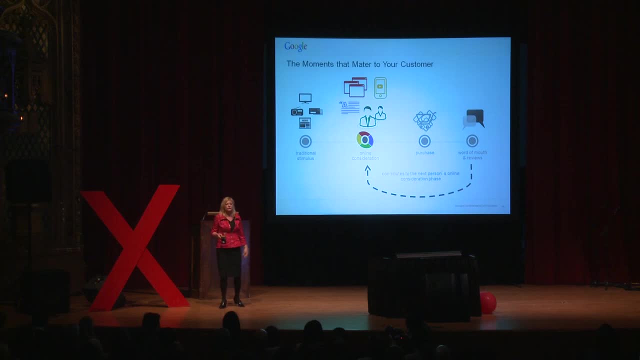 Marketers now have to win that moment of truth, in addition to the other places- And the majority still spend most of their resources against the traditional side of things- And online wins the moments that matter. So, if you look at this from awareness, familiarity, consideration, selection and loyalty, 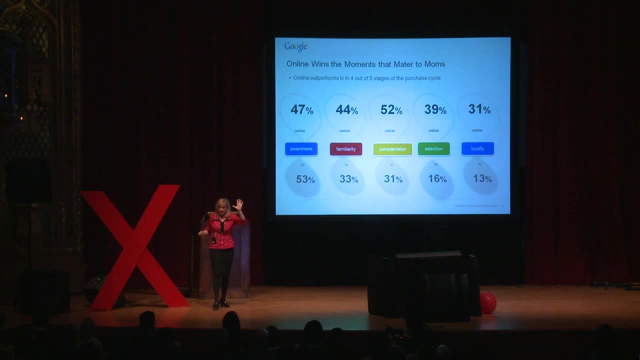 only TV wins in awareness. It's still important. I don't want to walk away saying no more TV. TV is still very important, especially from awareness, But you've got to win some of these other places that people are making their decisions. 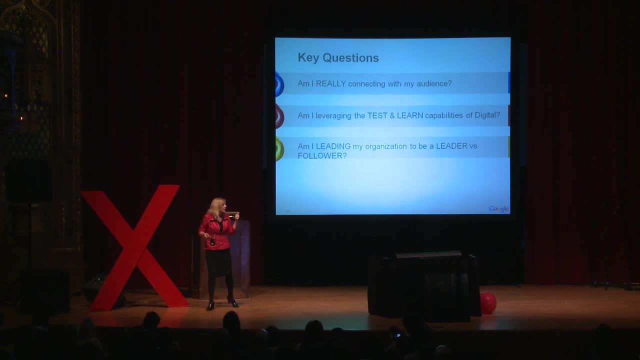 So I like to say: get going or get left behind. Am I really connecting with my audience? So if I'm a marketer, put my marketing hat on. Am I really connecting with them? You look at this TEDx group. They did a lot of marketing online to reach this savvy consumer. 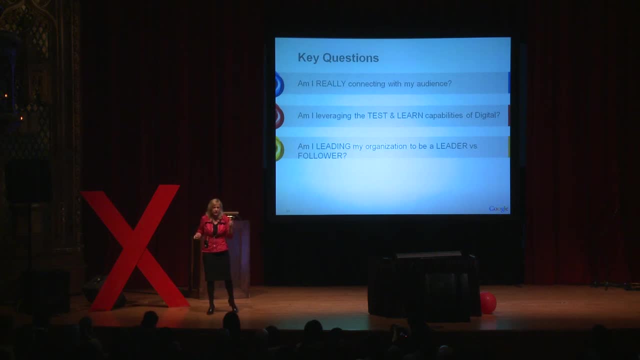 Am I leveraging, test and learn capabilities that are available to the digital Internet? In fact, it was really interesting. We have a new VP of marketing at YouTube And he came from Procter & Gamble, a very successful CPG company, And when Larry, our CEO, asked him, he said: 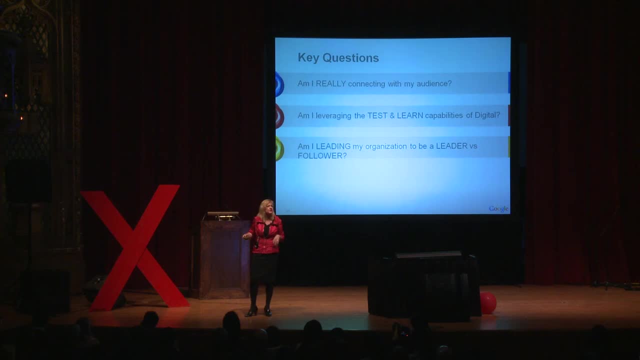 Lucas, what are you most proud of in your career? your successful career at Procter & Gamble? And Lucas said: hey, I always landed the plane. I ran 15 different brands, from Tide to Pampers, and I always landed the plane. 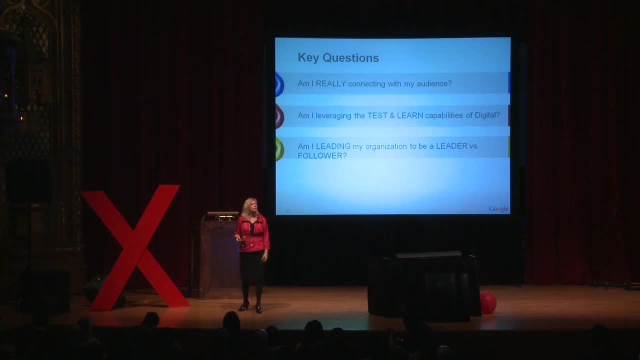 And Larry took a step back and looked at him and he said: well then, you obviously weren't taking enough risks, Really, Because that's the way we have to think today, and digital allows that. You can put messages out there, test them, pull them, learn from them. 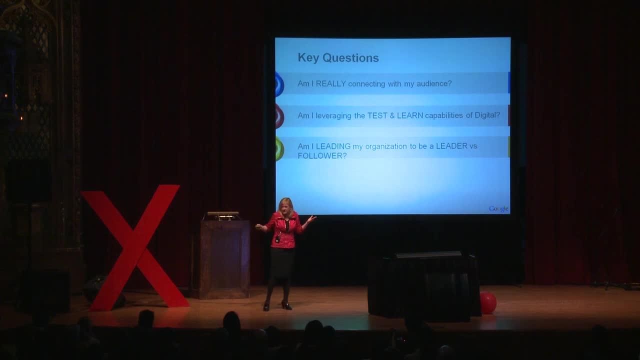 You don't have to be perfect. At Google, we call it fail fast And projects don't fail. We sunset them. And then am I leading my organization and am I teaching us to be a leader versus a follower? Back to my mobile example. 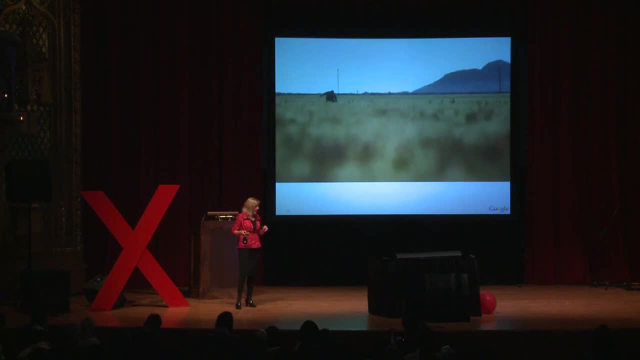 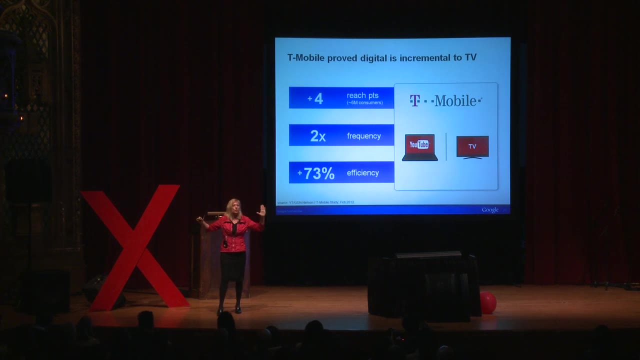 Oh, we'll get to mobile in 2014.. Well, good luck with that. We actually did a study of TV and the internet, So again I'm saying it's a yes and world. So when we worked with T-Mobile on a campaign, we did TV only in some markets, and then TV and video. 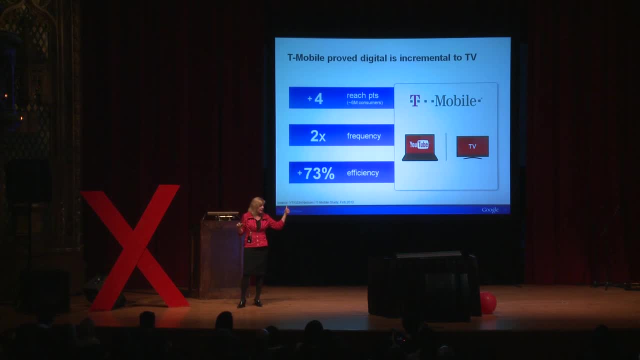 And in the markets where we did TV and video, we found a four increase in reach points, two times in frequency and 73% in efficiency. And that's important because, guess what? The internet is pretty darn efficient. You can be very targeted and it's a lot cheaper in most cases than running TV. 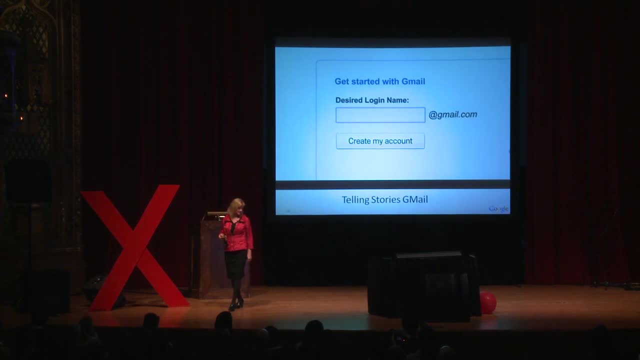 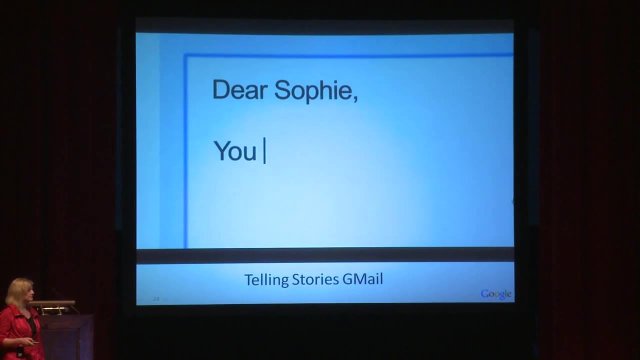 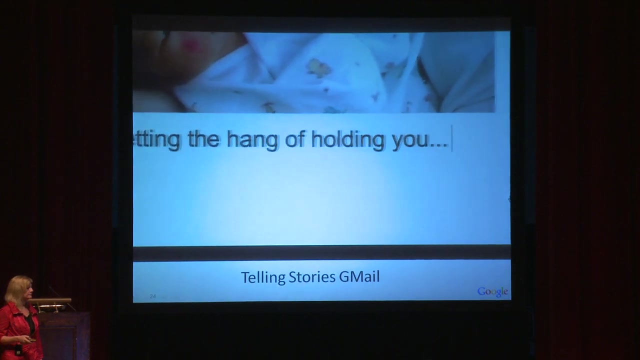 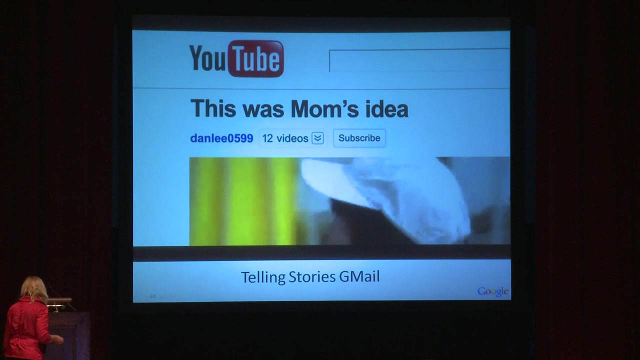 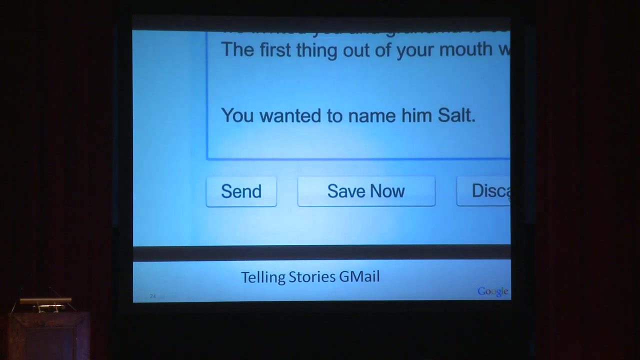 Are you ready for your big party today? Huh, The internet is not. Let's go. All right, I got everything. When I got you, it wasn't. Tell me what was it. What is it? Yeah, it's the internet. 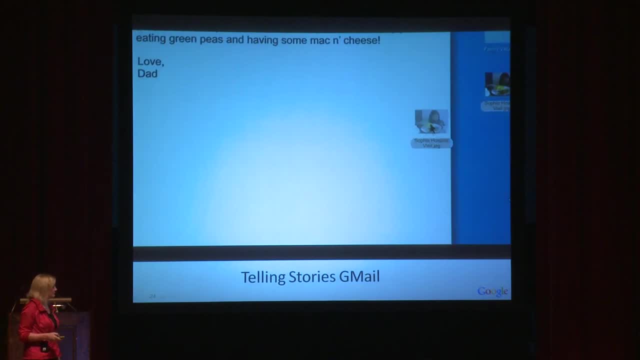 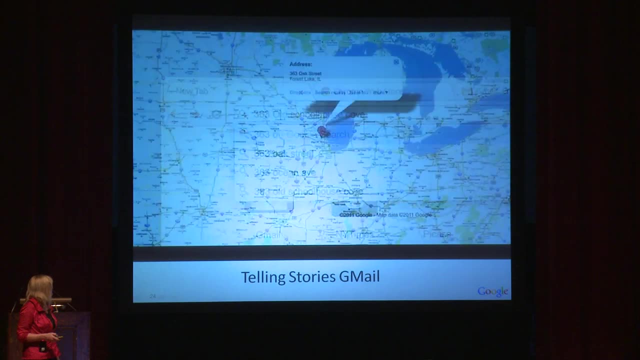 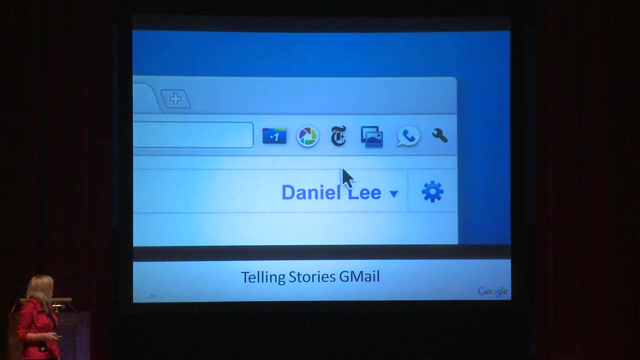 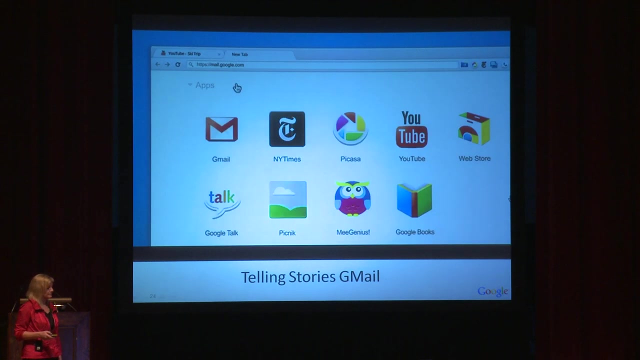 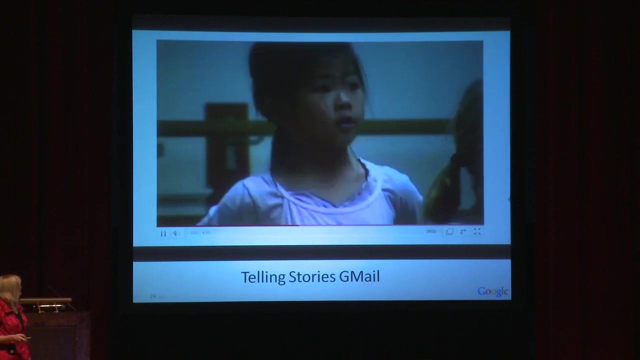 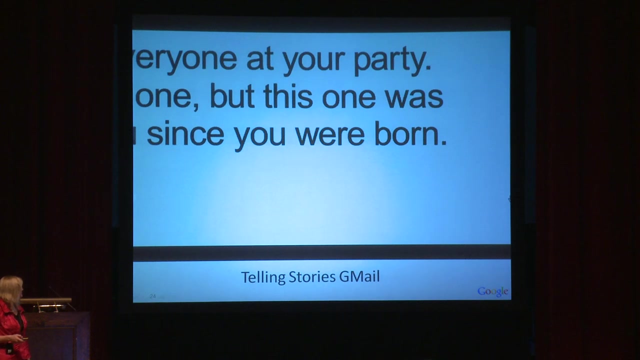 Where does the internet go? It goes across the internet forever. That's where you will learn to don't mess with my or my dreams at my desk. Wow, Yeah Well, you know, I don't know. So I was going to set up that video. 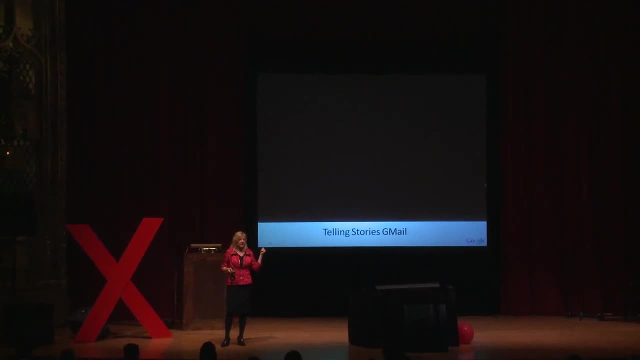 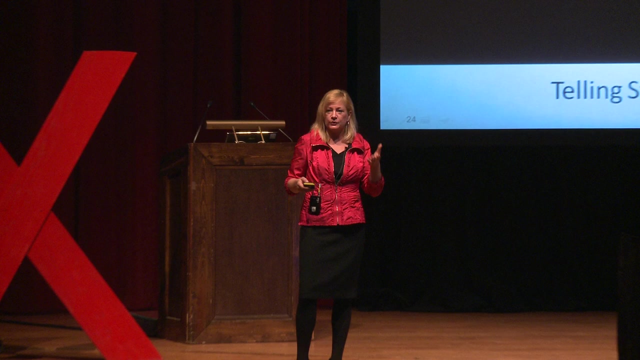 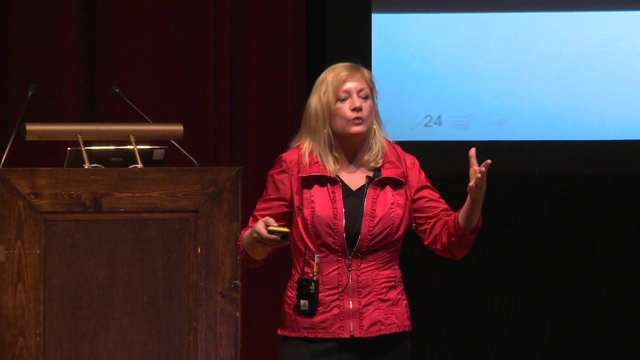 It clicked on very quick, But Daniel Lee is actually a Google engineer writing code out in Mountain View, And so that was a real-life story of what he was doing to connect with his young daughter, And I use that as an example of the way that Google View is advertising to a certain extent. 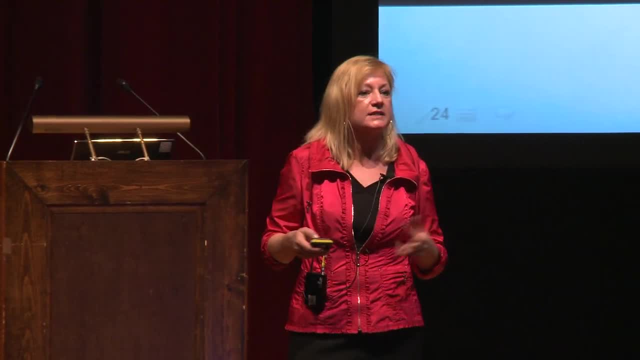 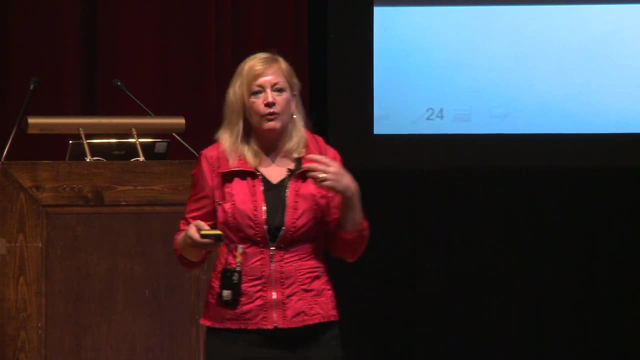 That's an online video ad, but it also has run on TV a little bit, And Google is a very big brand, but we don't necessarily advertise like a Chevrolet or a Coca-Cola. A lot of it is a little bit more subtle. 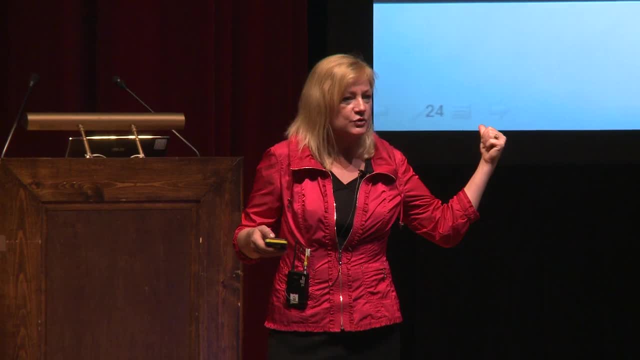 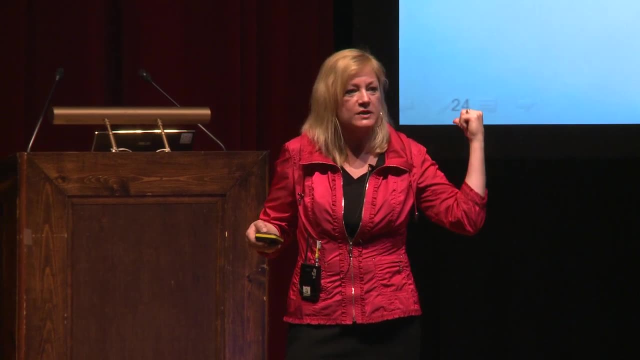 And really what advertising gets to is: it's all about the storytelling, It's all about the bonding, the engagement. So the insight is still just as important today as it was back in 71 when Harvey Gawar came up with: I want to buy the world a Coke. 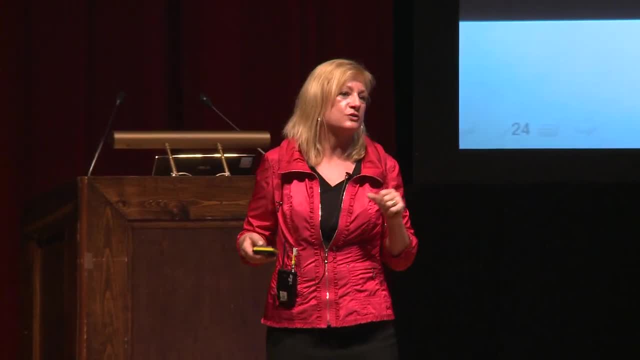 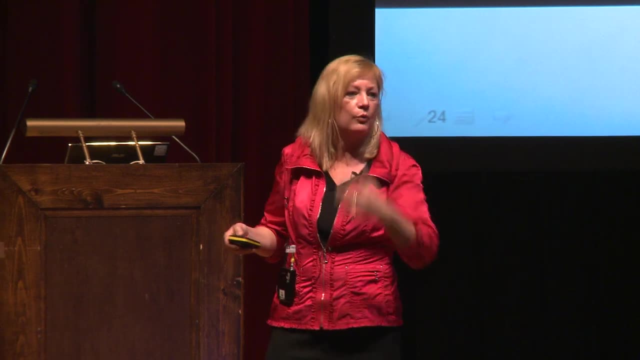 It's still very important, but the way to tell those stories is changing. And that's just an example of wow, this is how he's using Gmail. This is a great way for us to tell the world about. here's another way to use Gmail, for example. 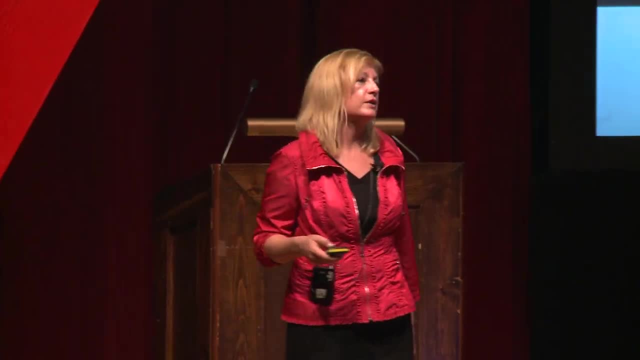 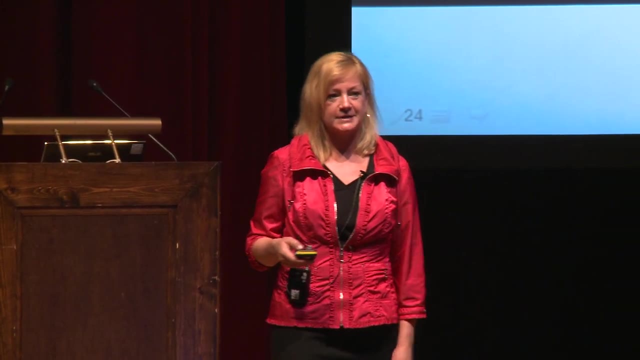 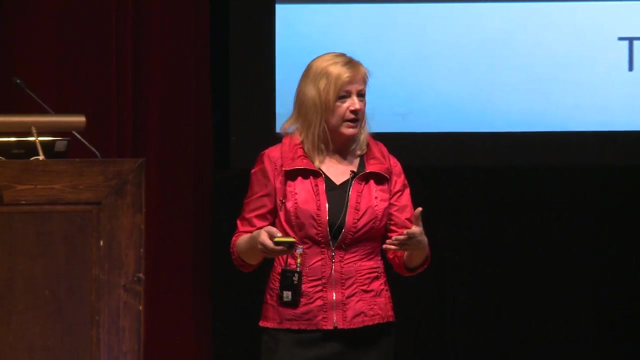 And I guess, lastly, what I would say is in working with a lot of our large advertisers, I met with one of the chief marketing officers for a major CBG company based in Cincinnati and he had his presidents around the table And we were talking about digital. 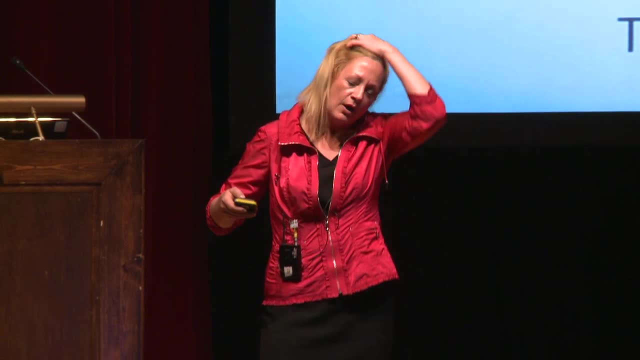 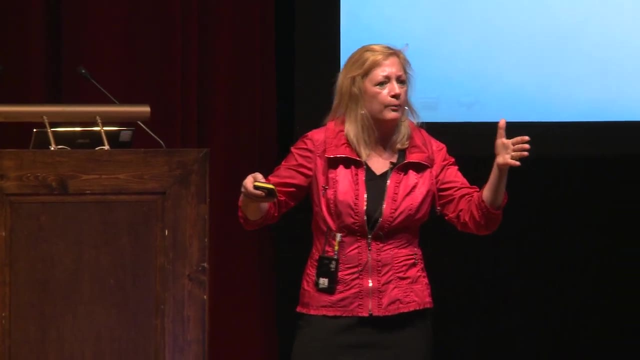 and they were coming up with all the barriers- And this is a couple of years ago, but all the barriers- of why they weren't doing more search, for example, or video or just digital in general, and why more budgets, even though consumer habits and time spent on TV 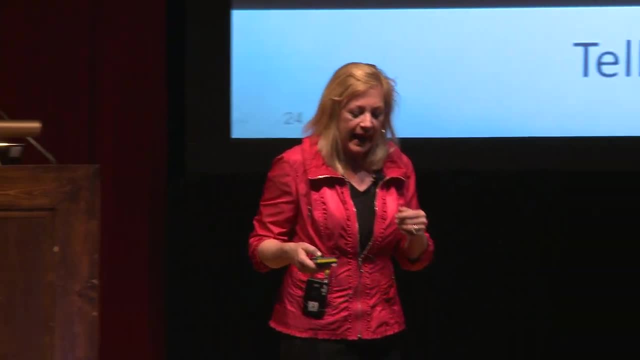 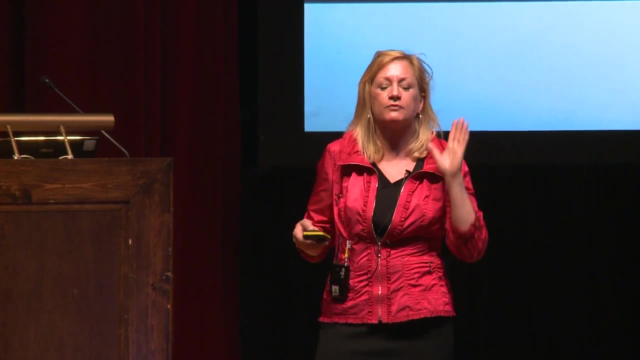 had shifted to digital, why they hadn't moved more in that direction And they had a lot of barriers. We can't measure it the same way. You can't use the same creative, You know. they just had excuse after excuse And finally he stood up and he was new in his role. 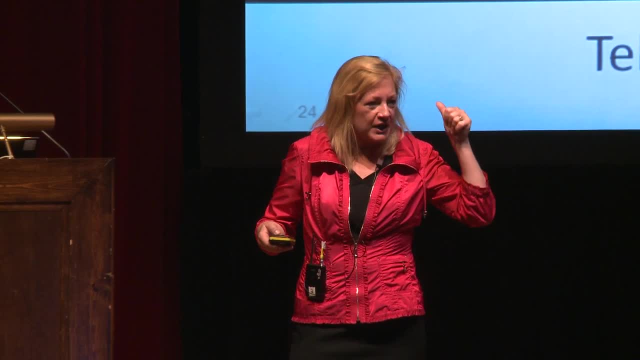 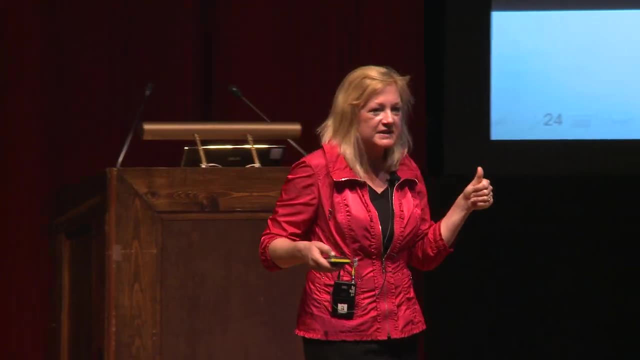 and he said we are at the forefront of a change in consumer behavior that we have not seen since the 1950s and TV. And in the 1950s and TV we didn't stand back and say, oh, let's be a slow follower and see if this thing sticks.